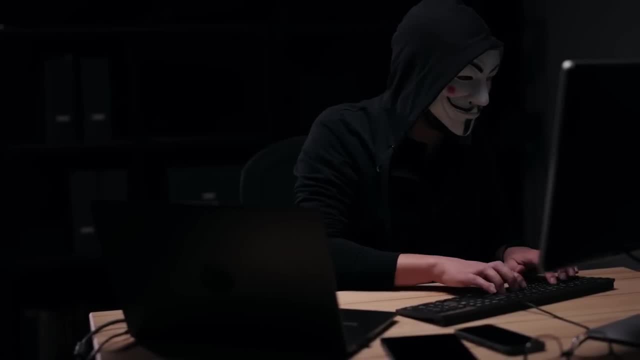 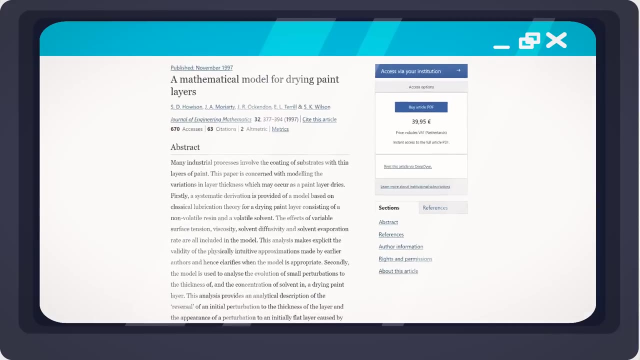 them. If I was a criminal, I would use one of the many, many sites online that lets you download academic books for free. For further research, I will head to Google, Scholar or JSTOR. This is where you can find academic research. 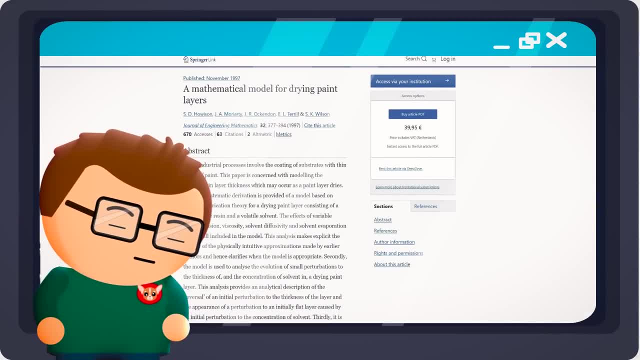 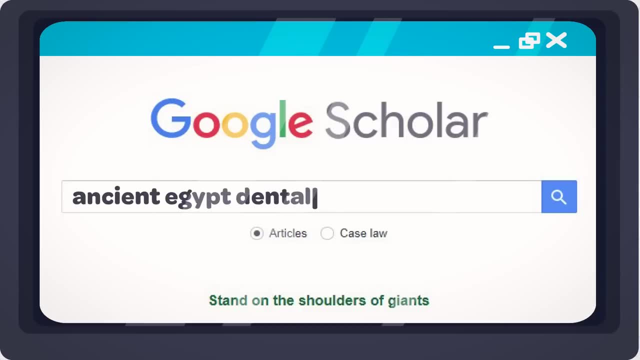 Which normally aren't the most fun to read, but they do have a lot of detail. Google Scholar is an amazing search engine. You can type in anything like, say, ancient Egyptian dental health, and you'll get an infinite amount of papers on the subject you 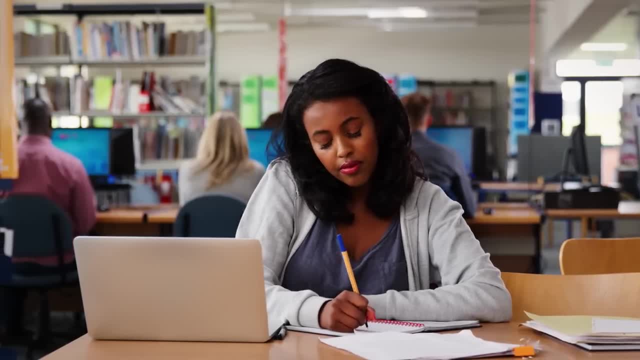 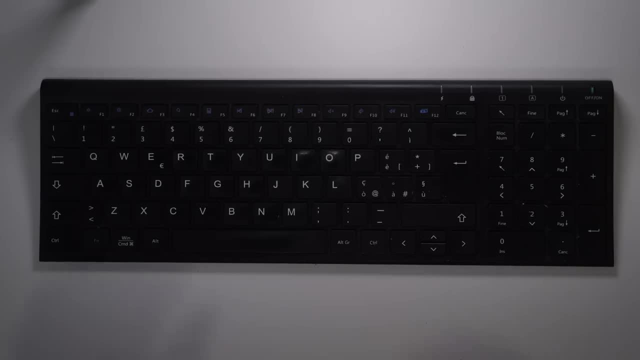 searched for. If you're in university, you probably already have free access to most of these papers. Otherwise you're going to have to pay for them Or if you email the author really nicely, they might send it to you for free. People of a sinful and criminal nature would probably go to. 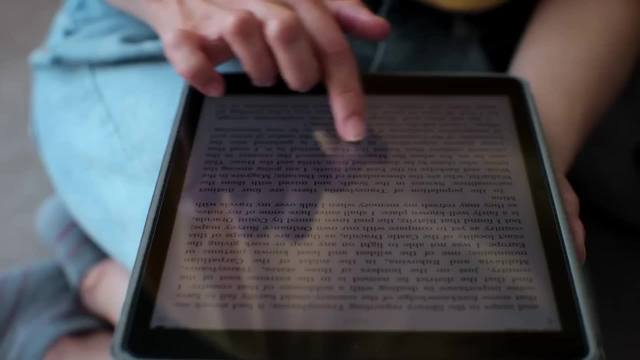 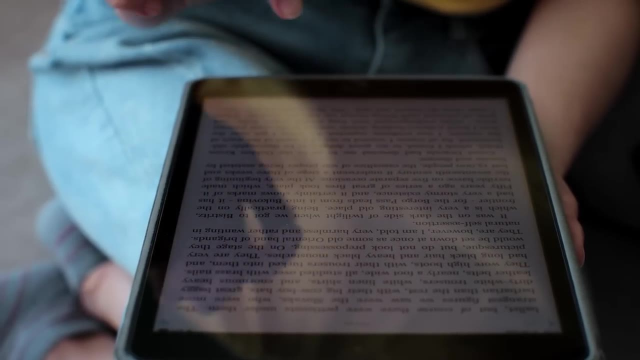 sites online that let you download academic papers for free. While reading books and papers, I pay close attention to their footnotes, references and bibliography. They are usually useful jumping off points for further research. If I find a really good book, I'll search the author's name and see if they've written anything. 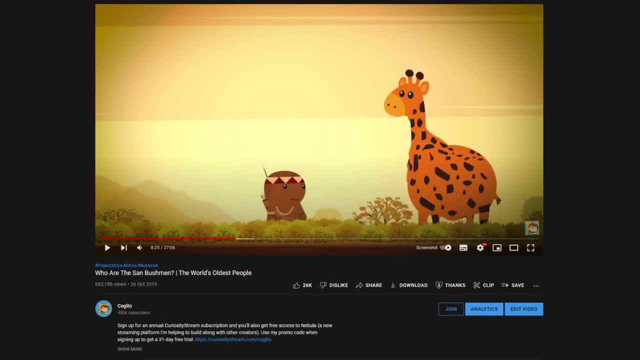 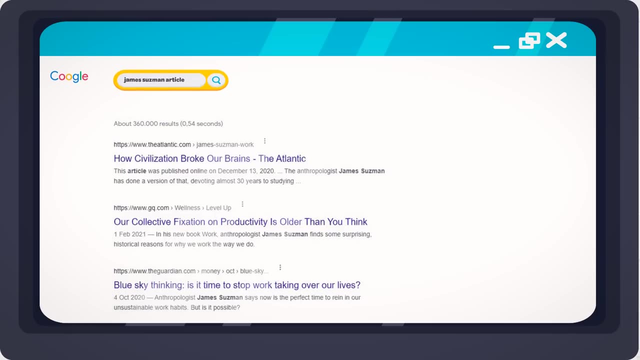 else on the subject. For example, when I was writing my video on the sand people, I read books by a guy called James Suseman and they were amazing. I searched his name on Google plus the word article and found dozens of articles that he had written, which helped a lot. 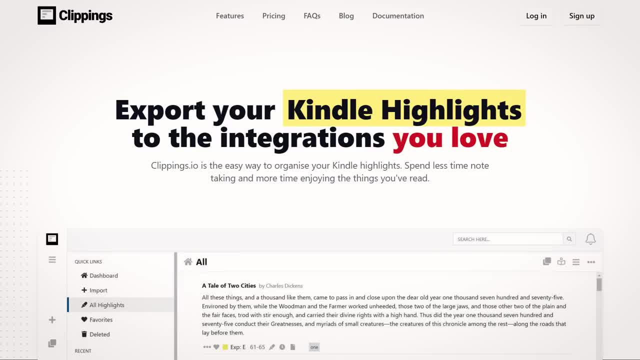 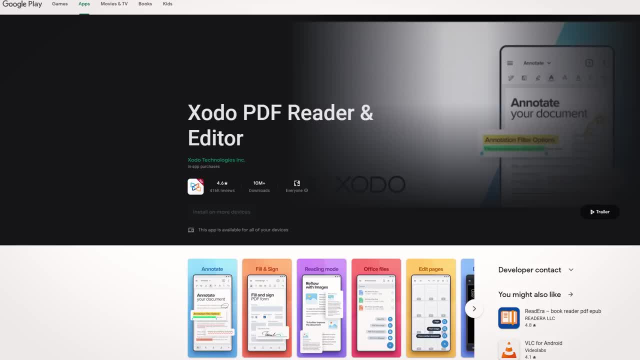 If I read something on the Kindle, I'll use clippingsio to export all of the highlights I've made while reading. If I did it on my tablet, I'll use Zodo Reader, which has a built-in highlight exporter. Once I have all my research, I'll open a Google Doc and start writing. I always 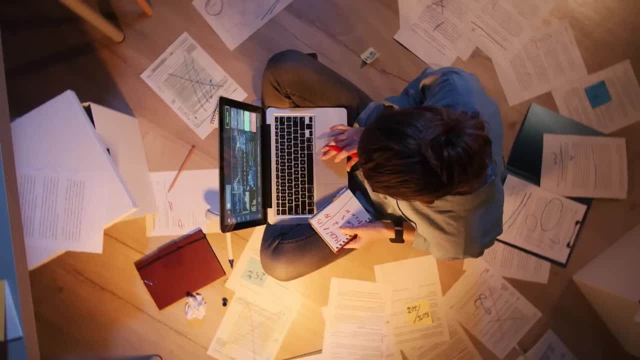 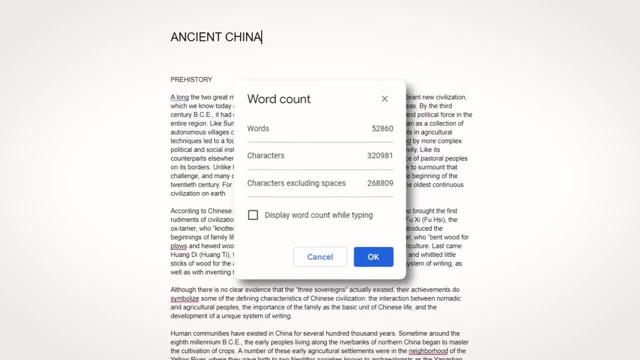 write with my thousands of words of research notes nearby so I can check them constantly. For example, this research document from my video on ancient China is 52,000 words long. It has direct quotes from books, random notes from me, pictures, maps and. 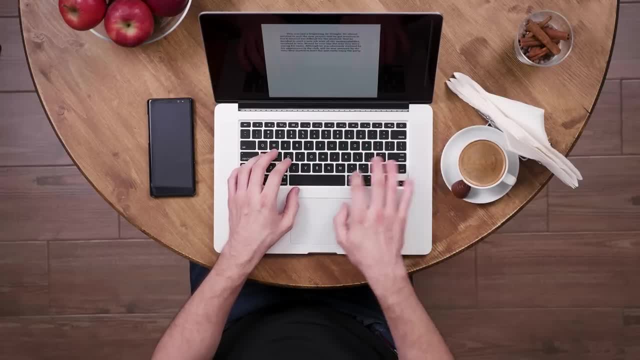 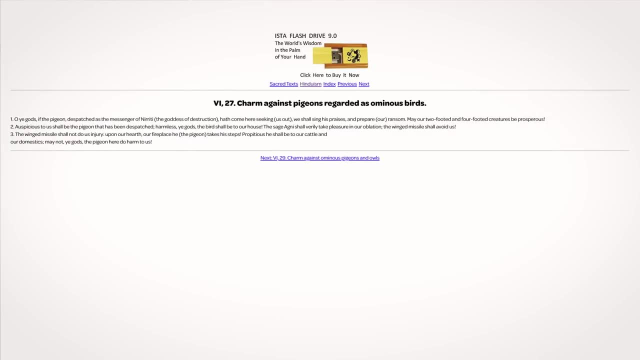 An entire section just called Red Pandas. With my script skeleton in front of me, I'll figure out the key pieces of information I need from all of my research. So if I'm writing a script on Hinduism and I read one of the Vedas and highlighted an important passage, I'll grab that highlight. 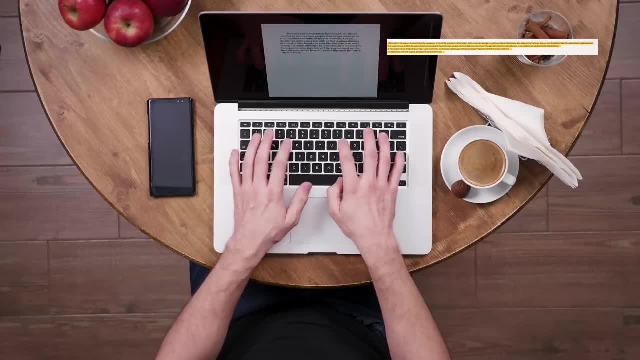 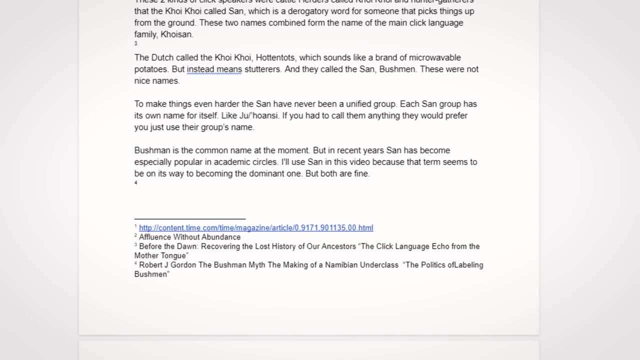 see if it helps explain the point I'm trying to make, and then I'll figure out if I just quote the passage or if I summarise it in my own words. in order to back up my explanation, I like to put little footnotes in my scripts as well, so later on I can see where I actually got that information. 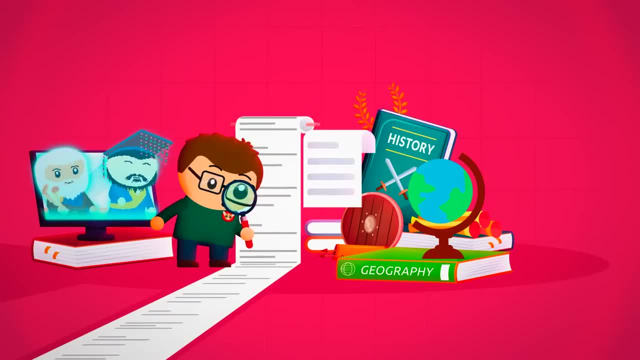 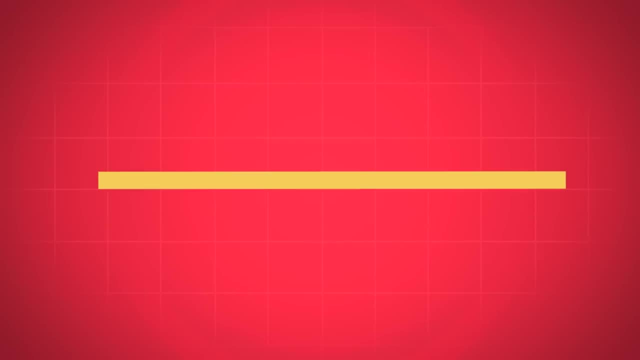 Every point must be backed up by research and sources. I simply rephrase what the sources say. A lot of the time, research notes that were thousands of words long turn into just one sentence. We recently brought in a researcher slash writer. that has really helped this whole. 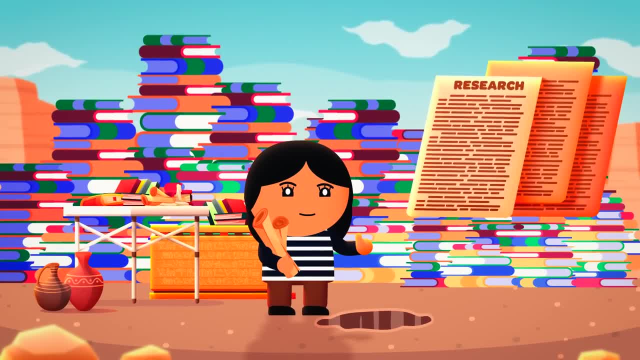 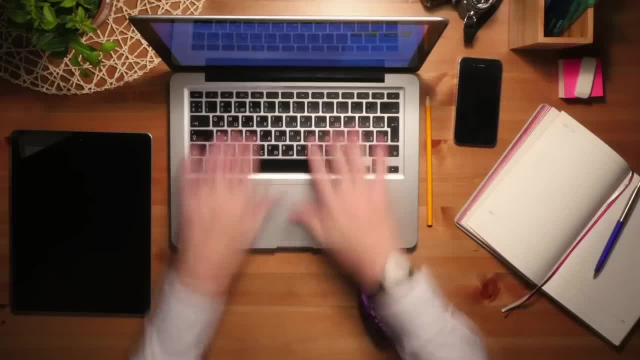 process. We were incredibly lucky to find someone as talented and intelligent as we did. It has improved our videos by 1 million percent. Look, I made a graph that proves it. Once the script is written, it's usually way too long By like. 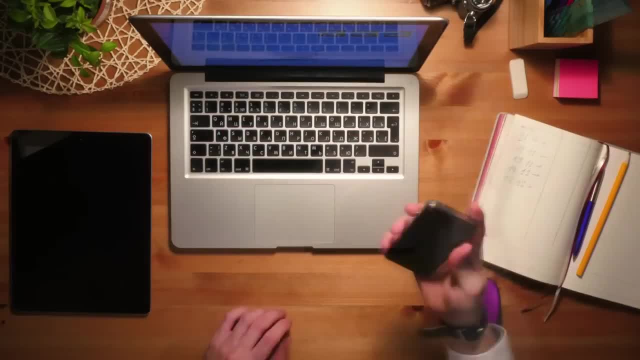 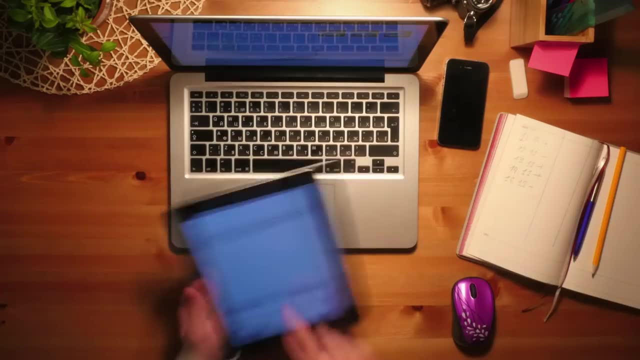 several thousand or tens of thousands of words. This is when the cutting process begins. My entire goal here is to make every single paragraph or line shorter and clearer. I'll slice through the script, cutting out whole sections- which is painful- until it's just a few thousand words. 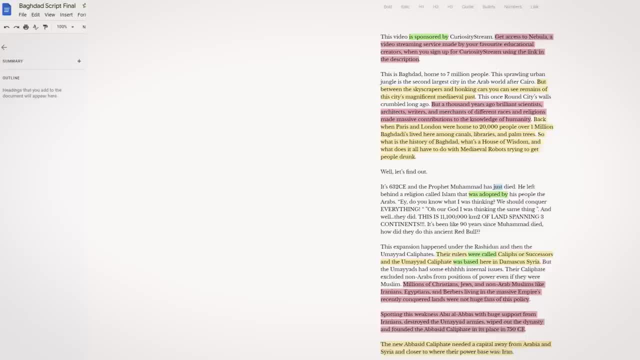 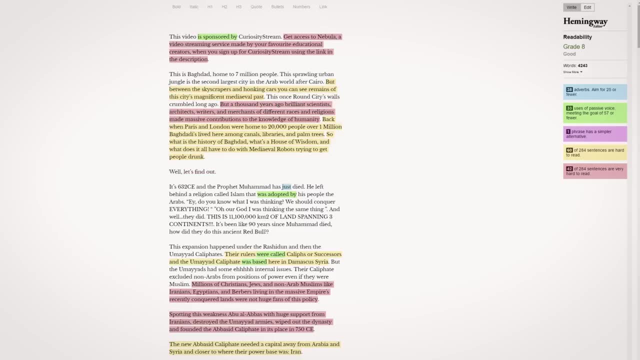 too long, Then I'll bring it into an app called Hemingway Editor, which you can use for free online or you can pay to use it on your desktop. This app highlights long, complicated sentences and wording. Using this, I rewrite every sentence until they are. 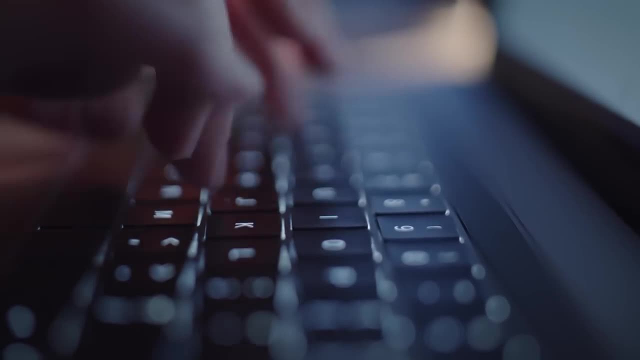 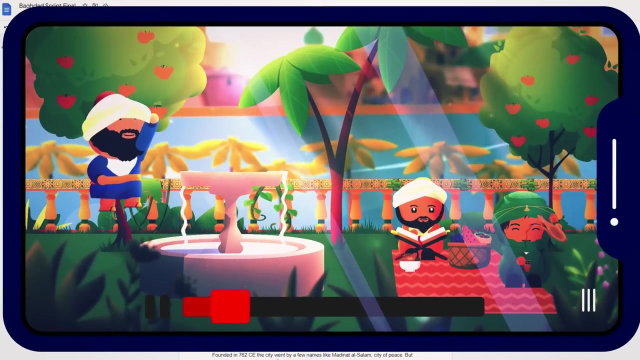 short and as clear as possible. After weeks of researching and writing, I'll have a script that floats between 2,800 and 4,000 words. Because I animate everything, I need the scripts to be around 20 minutes or shorter, because otherwise it would take forever to actually finish a video. 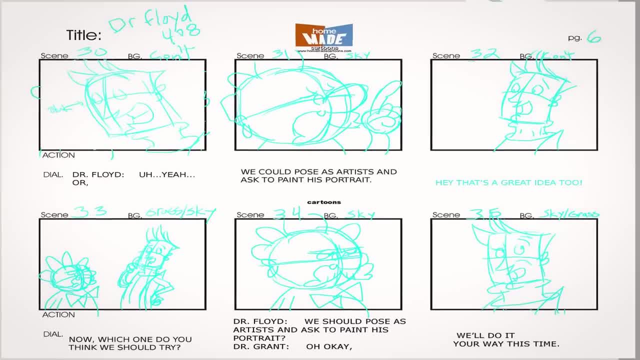 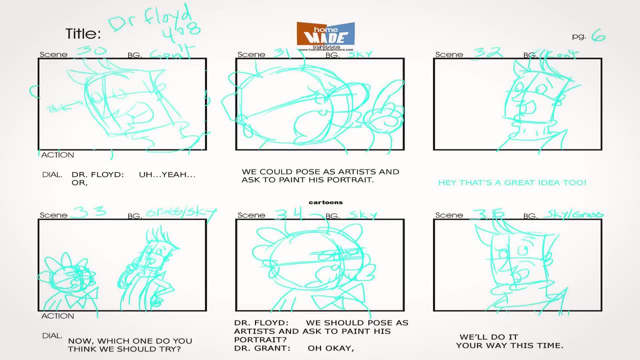 Once the script is done, it's time to storyboard it. A storyboard is just a series of really quick sketches to let me know how every scene needs to be animated and what scenes or characters I'm going to need our illustrator to draw. What I do is create a huge 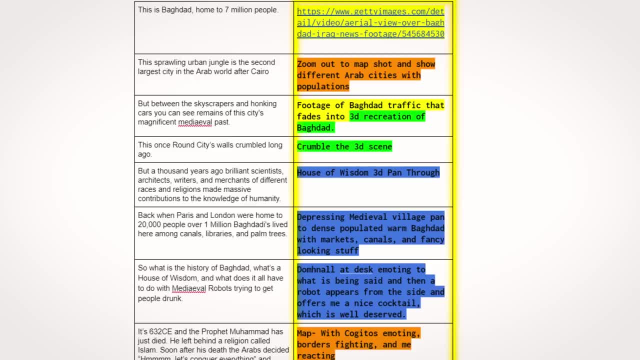 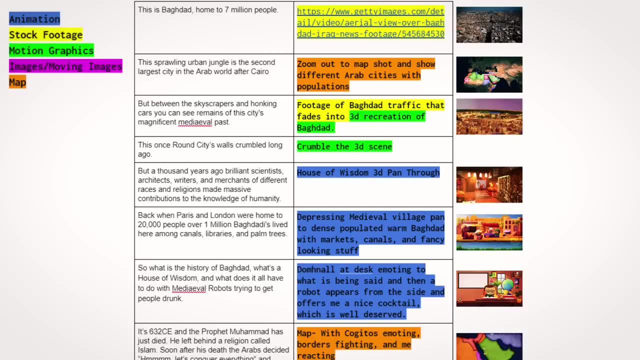 table in a Google Doc. One column has the script. the next column has a description of what will happen on screen. while I read that part of the script, I colour, highlight everything to make it easier, and so I can see if there's too much of one kind of animation. 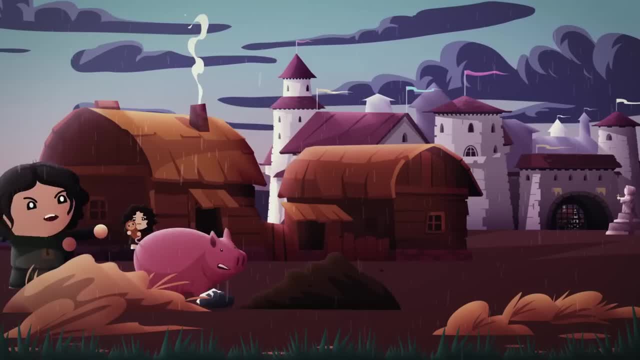 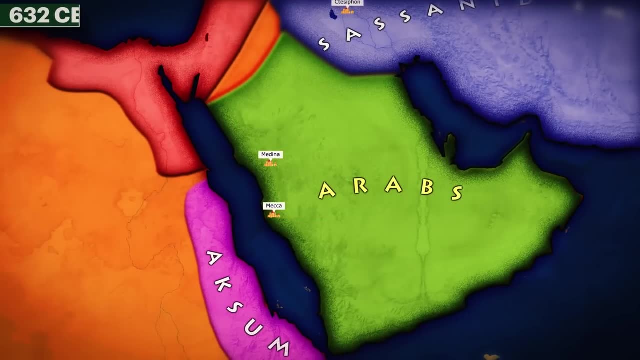 My colours are for: 1: animation, which is like the traditional 2D scenes with characters, 2. motion graphics, which is when I animate words, graphs, anything that's not character based. 3, maps, which is for maps, 4, images, which is for images, and 5, stock footage, which 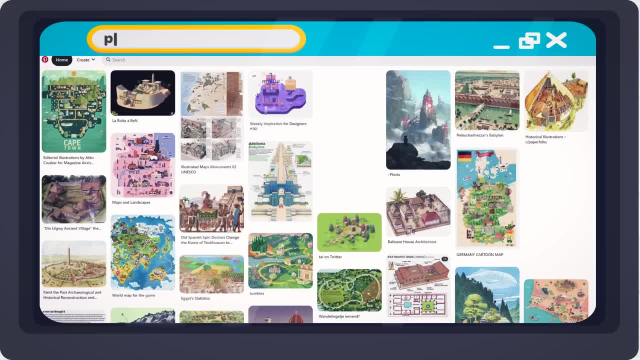 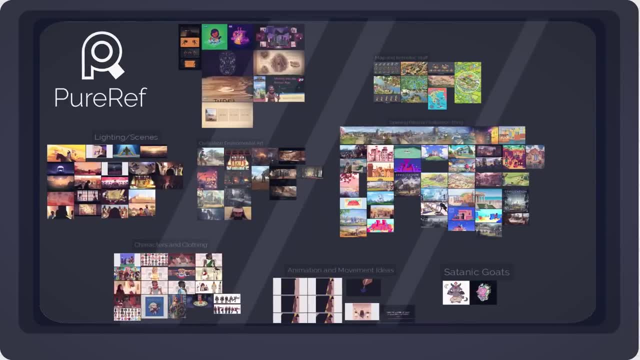 is yeah. When I'm creating my storyboards, I'll go to websites like Pinterest, Vimeo and Behance to collect some visual inspiration. I'll save all these shots in a free program called PureRef and use them as reference for creating my own scenes. 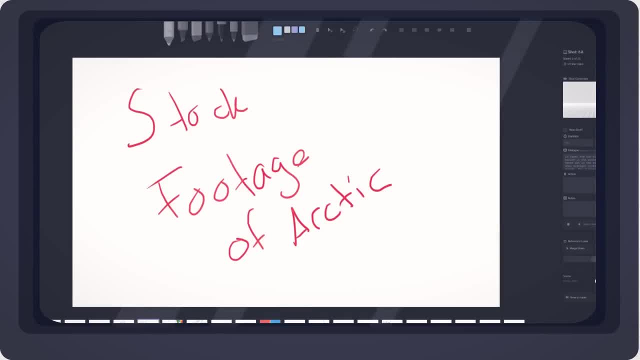 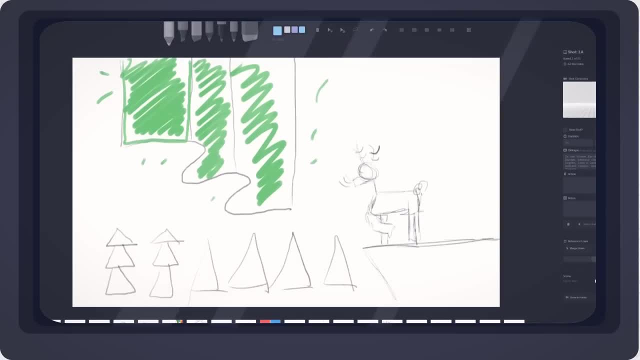 Once the basic storyboard is done, I'll do a fairly basic visual storyboard to see if things work. Sometimes I'll use an amazing piece of software called Storyboarder, which is free, where you can sketch out each scene with the narration in the box next to it, Or I'll just do something quick. 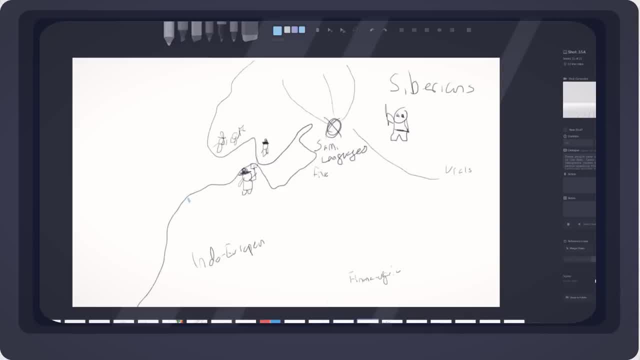 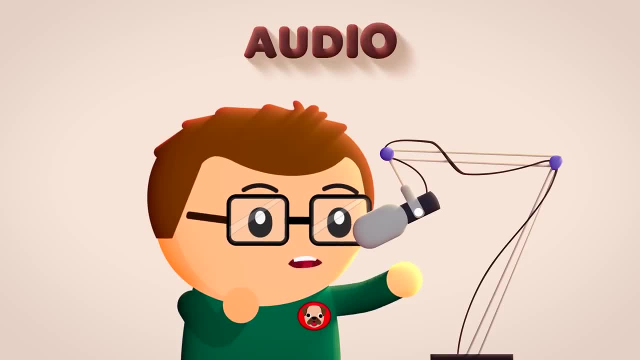 in Photoshop. These are just really rough sketches and sometimes I just write words or even just stock footage when I'm feeling lazy. Here's an example storyboard from my video on beer Audio. Once the script and storyboard is done, I'll record the narration. I do this after the storyboard. 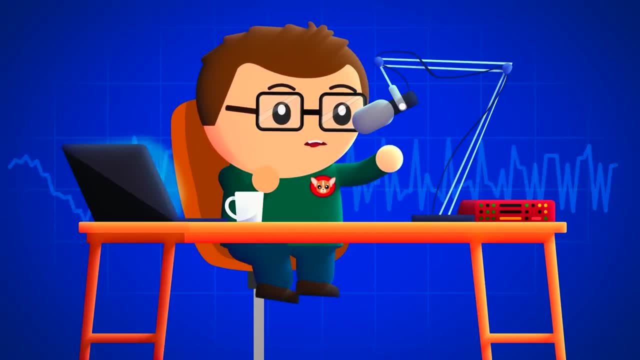 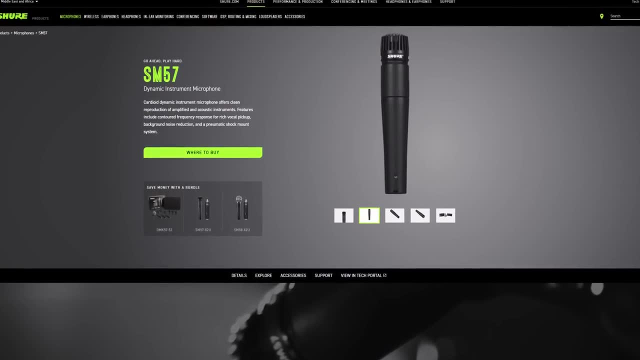 because sometimes I think of a scene while storyboarding that could be improved by narrating that scene differently. I record my audio on the Shure SM57LC microphone. It costs 105 euro. I bought it because apparently the audio quality from this microphone is the 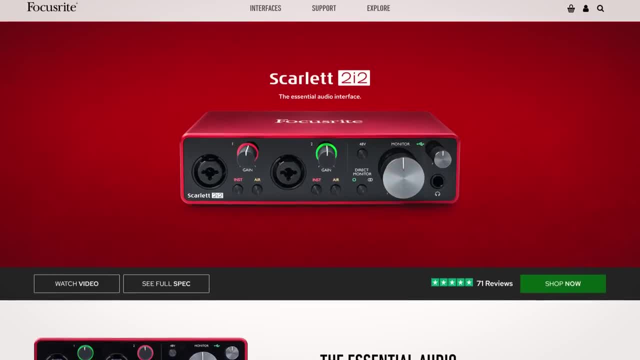 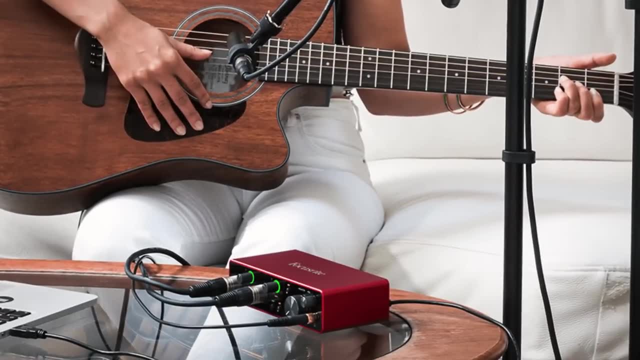 same as microphones, double and triple the price. You do need this expensive piece of equipment called the Focusrite Scarlett 2i2 to make it work, which costs 149 euro. You plug the microphone into the magic box and it makes my voice appear on the computer. Why do I need the box? I have no idea. 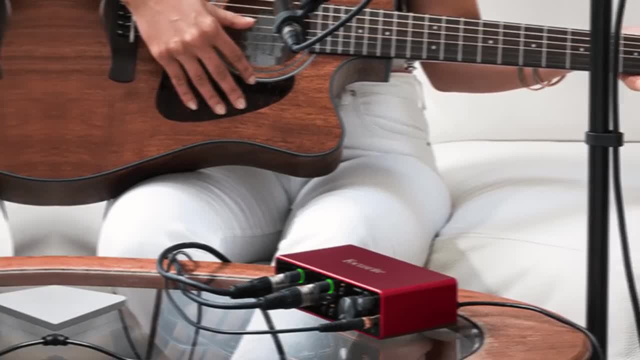 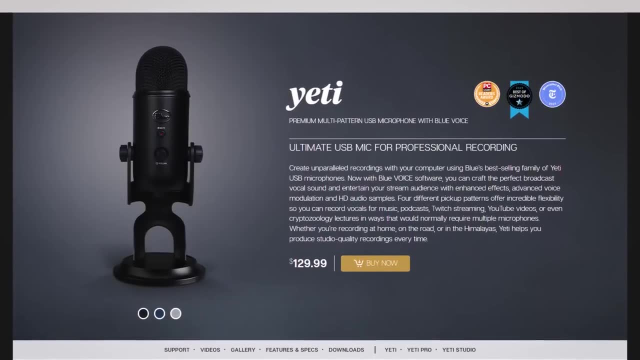 I am not a sound scientist, but if you don't have the box, the sound doesn't work. Before I had this kind of expensive setup, I used a $100 Blue Yeti which you just plug straight into your computer. My amazing wife built this recording box for me. I'm not sure if you've. 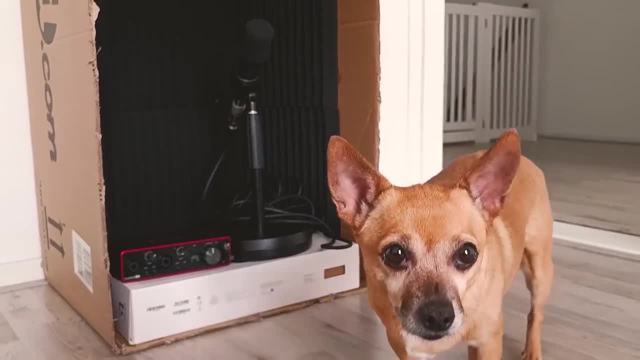 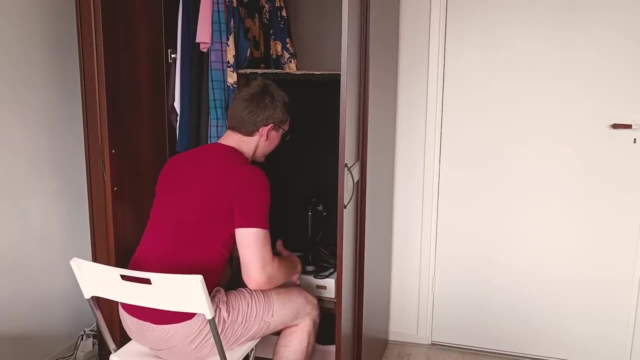 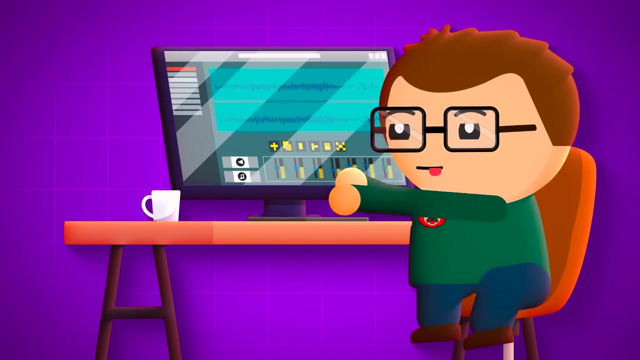 heard of it, but it's a nice little box to improve the narration quality. I place the microphone in the box, put the box in the wardrobe and then I yell at it. If a video is 20 minutes long, the raw narration for it is about an hour or longer, because I'm 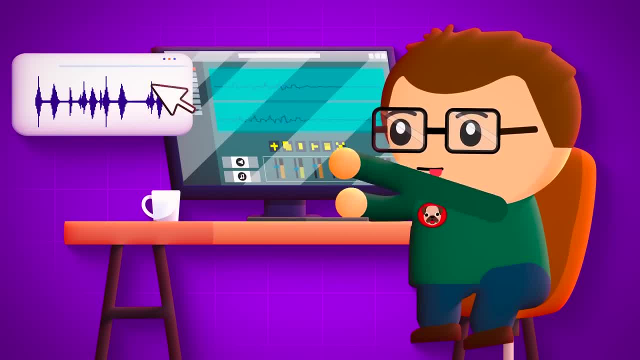 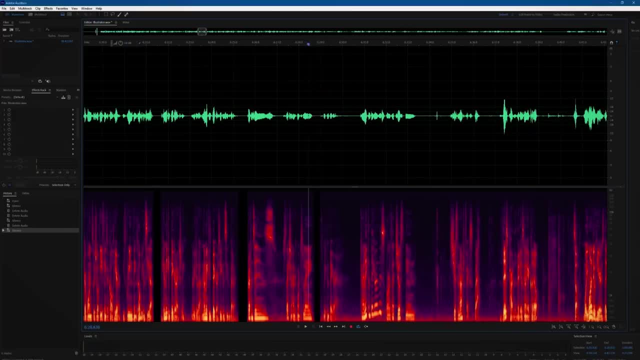 super not eloquent. Once I have that audio, I cut out all of the different takes the mouth clicks, the nasty breath noises and then throw on some effects to make me sound cooler. I do all of my audio editing in the program called Adobe Audition, which costs money. 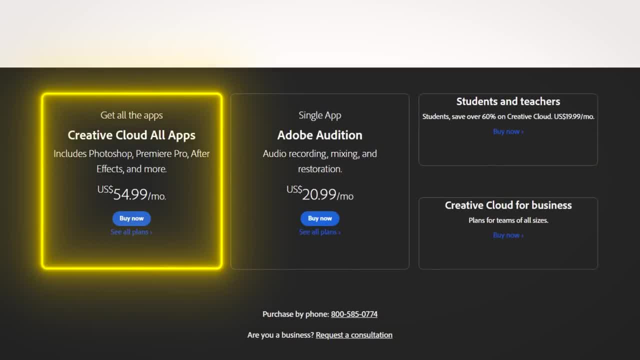 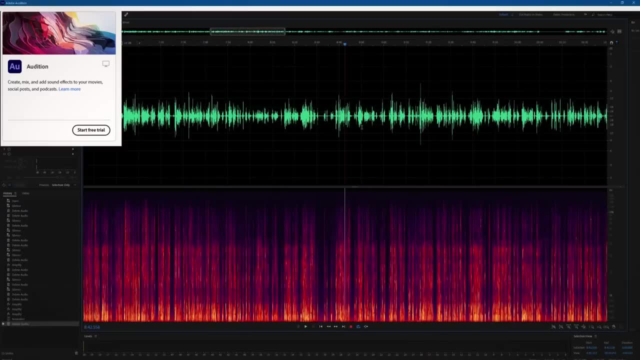 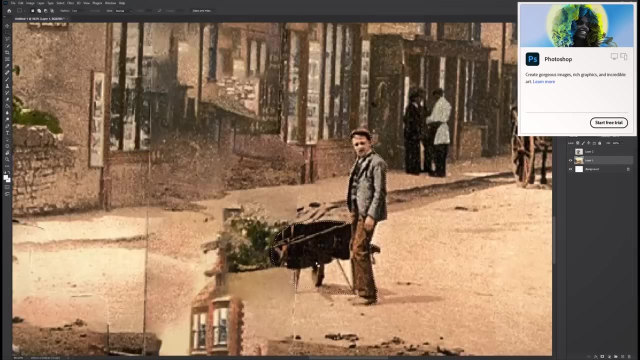 I'm subscribed to a thing called the Adobe Creative Cloud, which costs around 60 euro a month. This subscription gives me access to all Adobe products which I use for everything: Audition is for editing audio, After Effects is for animating, Premiere is for video editing and Photoshop is for image manipulation. I didn't always have this. 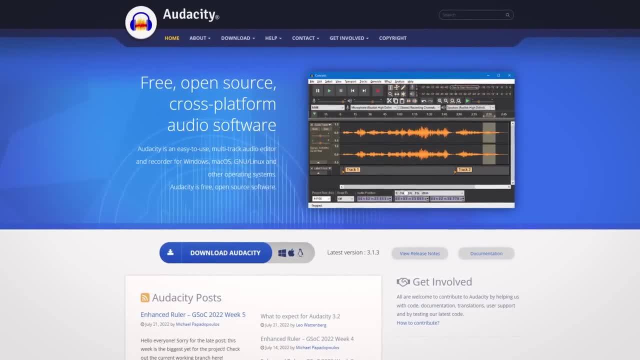 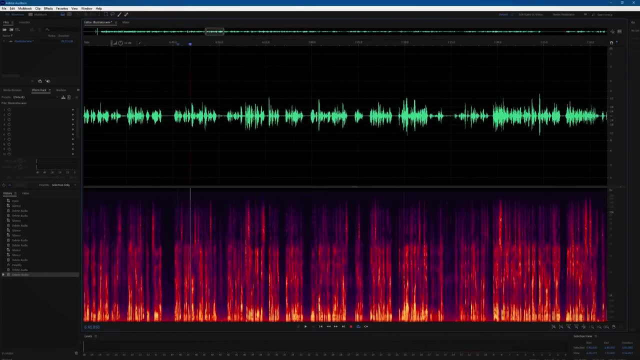 When I started out, I used Audacity to record and edit audio, and that's free and really good. Both Audition and Audacity have tons of tutorials online. They're easy to learn. Illustration: Once the audio is done, I start illustrating all of the assets that I'll need for the video. 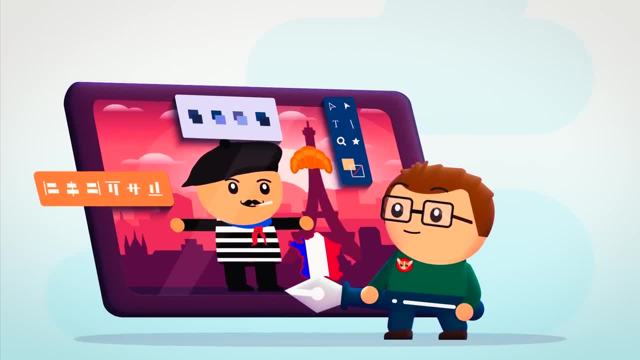 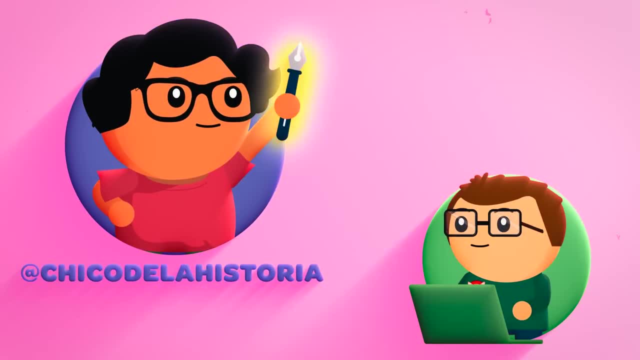 This includes characters, props, backgrounds and little icons. Before I did all of this by myself, but for the last video and for future videos, I have hired an extremely talented illustrator to help out with some of the illustrations. To make my illustrations, I use Adobe Illustrator. 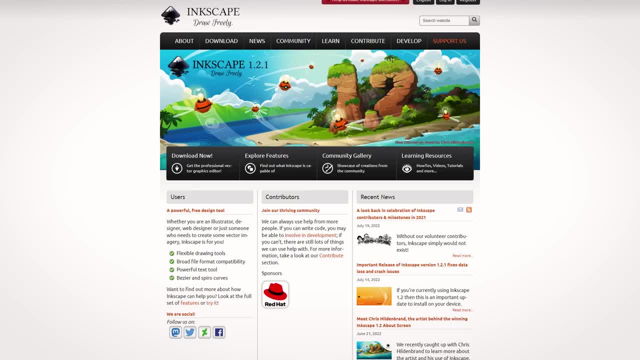 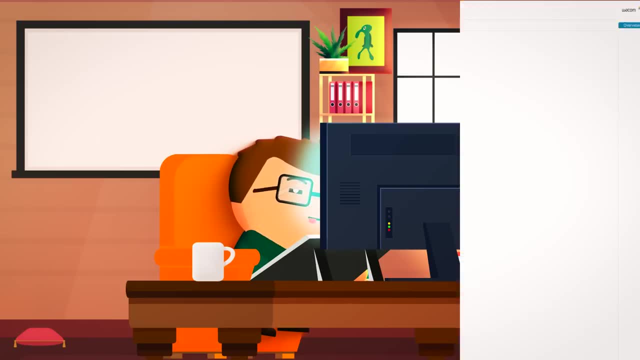 which costs money. but when I started I used Inkscape, which is free. You can draw everything with a mouse- I did for years- but a drawing tablet will make life a lot easier. Now I use the 350 euro Wacom One, but for years I use the much cheaper 80 dollar Wacom Intuos. 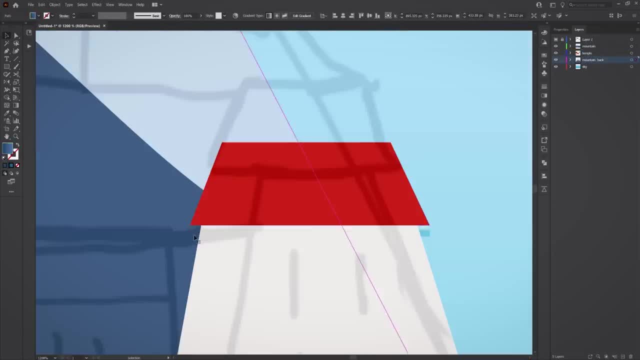 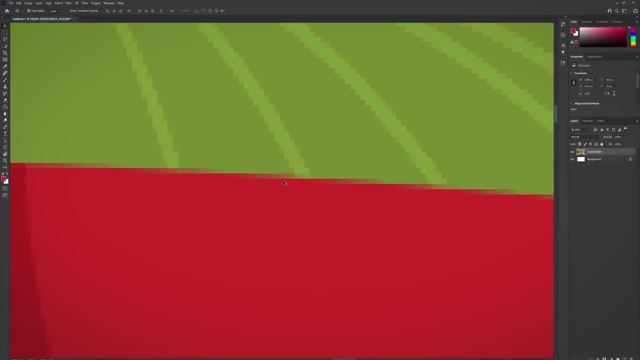 Adobe Illustrator is different to say Adobe Photoshop or the free alternatives, Paint or Gimp. Photoshop is raster based, which means it draws with pixels. That's why when you draw something in a raster program and then try and make it bigger, it gets blurry. Illustrator uses vectors. 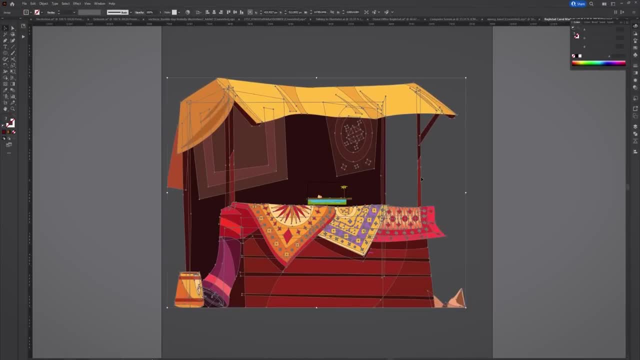 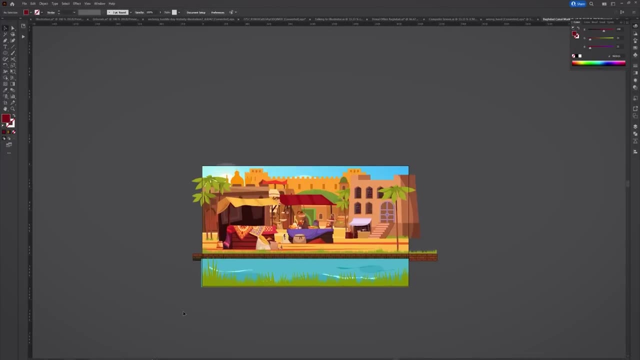 I don't know what that means, but if you make a vector drawing, you can simply resize it to any size and it stays sharp. That's why I use vectors for my videos, and most motion graphics you see will be vectors as well. Kurzgesagt is entirely drawn in Illustrator using 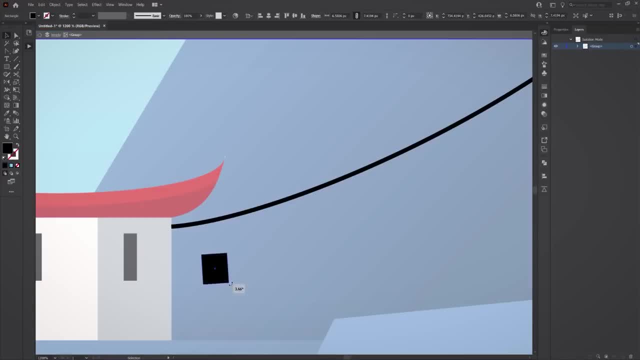 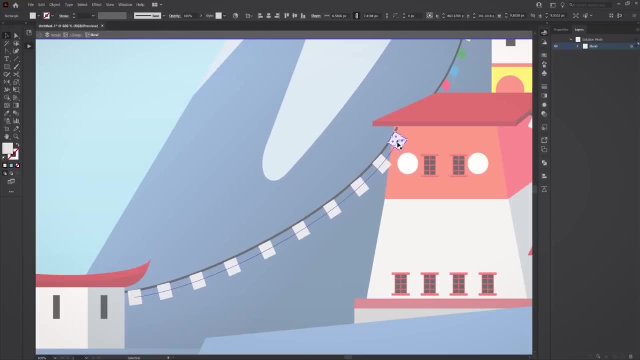 vectors. You can make anything in Illustrator using basic shapes. You don't need to be an amazing artist to get good results with this program. I know this because I can't draw, but I can use Illustrator. Here I'll make a character to show you how it's done. A circle for the head. 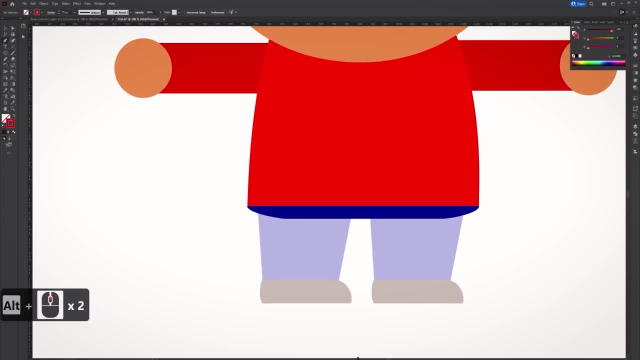 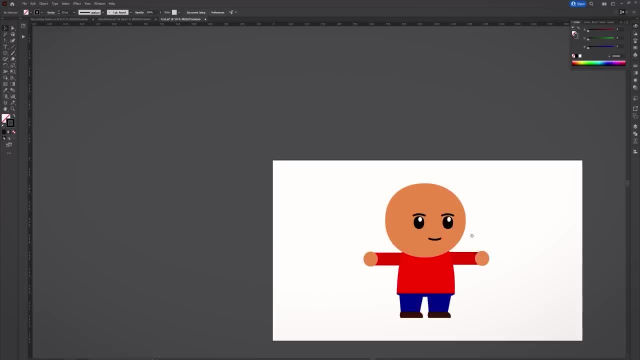 a tapered square for the body, straight lines for the arms, a tapered square for the legs, a rounded square for the feet, some ovals for the eyes, some rounded lines for the eyebrows and the exact same thing for the mouth. They're all extremely basic shapes that anyone can draw. I have a whole 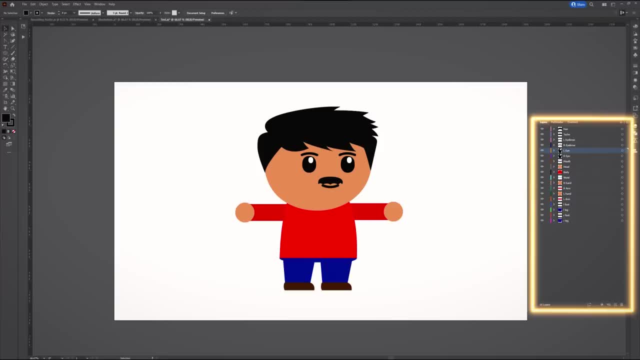 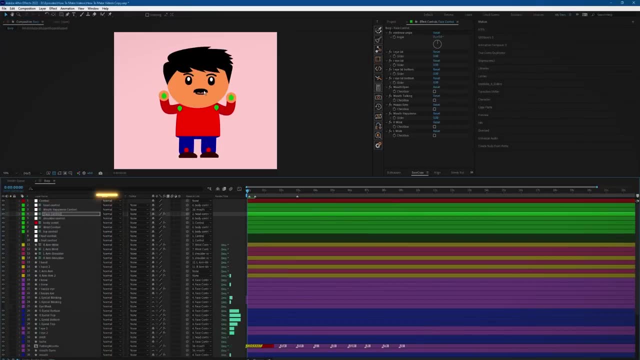 library of character assets here that I can dress them with. I label every layer with a clear name because when I bring this character into After Effects later on, the layers will appear as they were in Illustrator. So being organised at the beginning will save you a lot of time later on If I need to edit a real image or 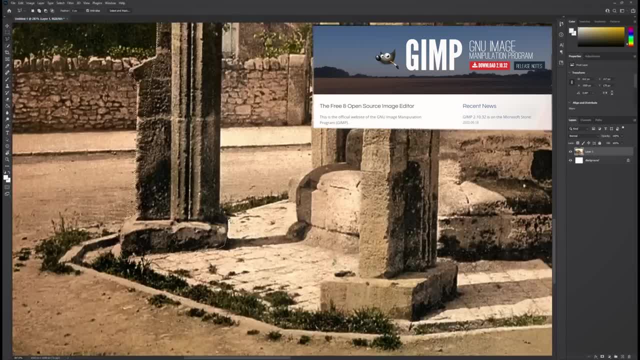 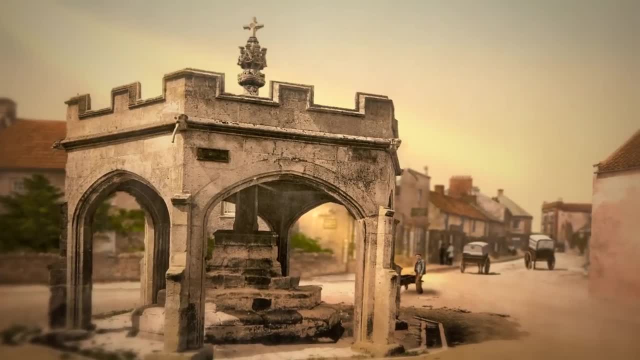 I use Photoshop, which costs money, but Gimp is free and is a really good alternative to Photoshop. I usually only edit images when I want to cut something out or make a cool fake 3D effect. To do this, I use the lasso tool to cut every part of the image out that I'll need to move. 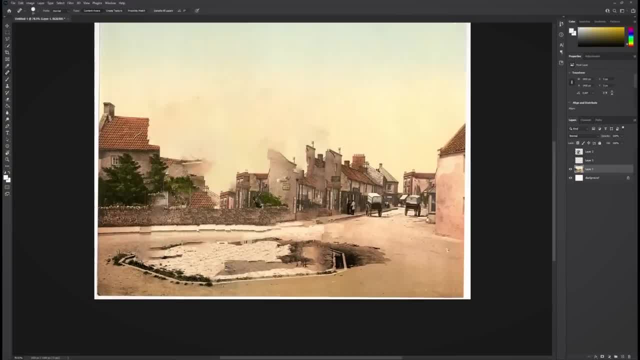 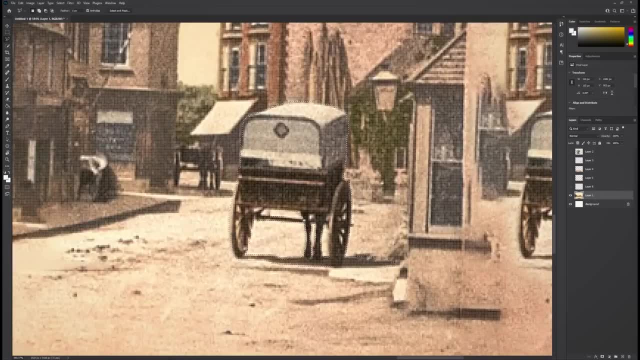 Mostly the foreground, midground and background. I cut them out, put them on their own layers and then I use the content aware fill tool to fill in those empty spaces. This tool is magic. I have no idea how it works. I can then bring those layers into After Effects. click this. 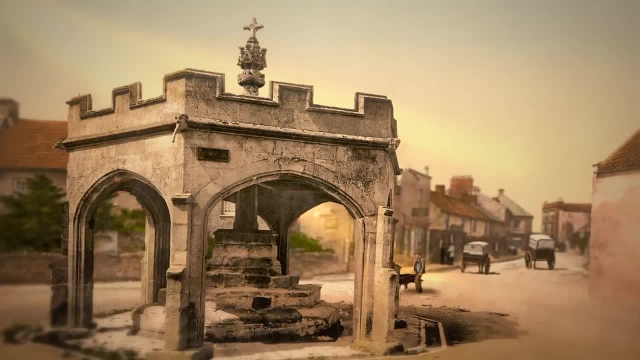 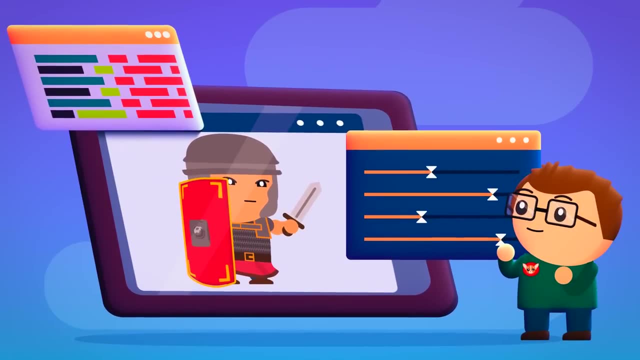 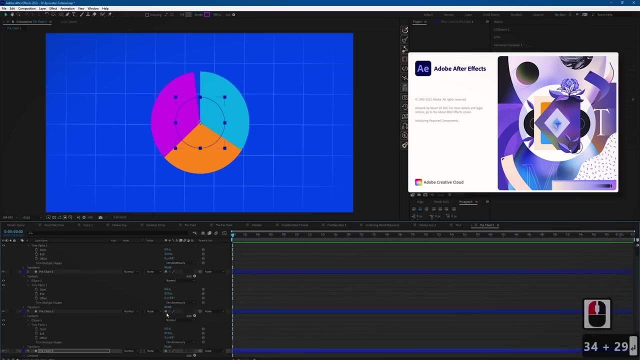 3D box, move the layers in 3D space, plop in a camera and now you have a fully 3D photograph- Animation- Ok, so here is the second most time consuming part of the video making process. I animate everything in this program called Adobe After Effects. It is an extremely powerful and extremely 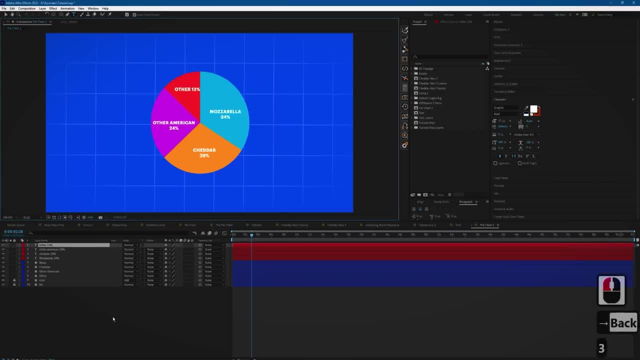 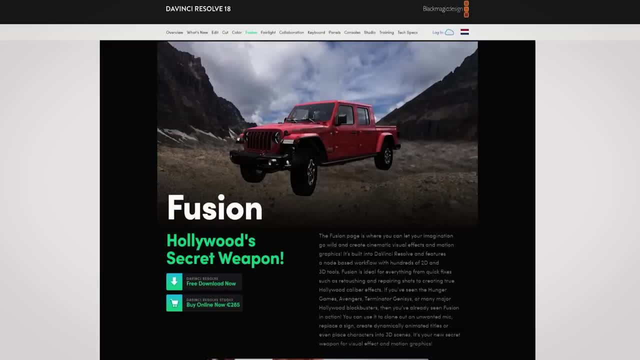 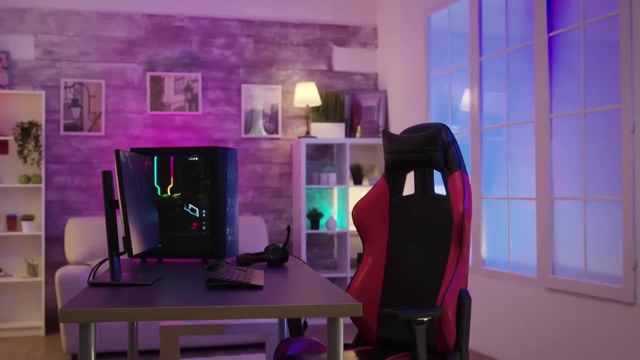 Other turnitves to Adobe After Effects are Gabillary and DaVinci Fusion. I haven't used them, but I have heard good things. Like I said, after effects are a pretty slow program so you'll need a decent computer or laptop to use it. Now, back in the day, I've used Ulkaly Deputy For the last few years, up until. 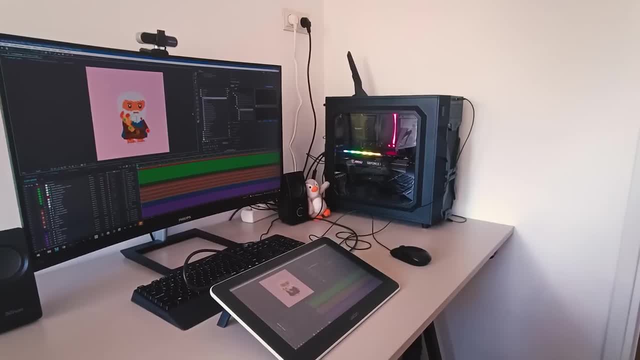 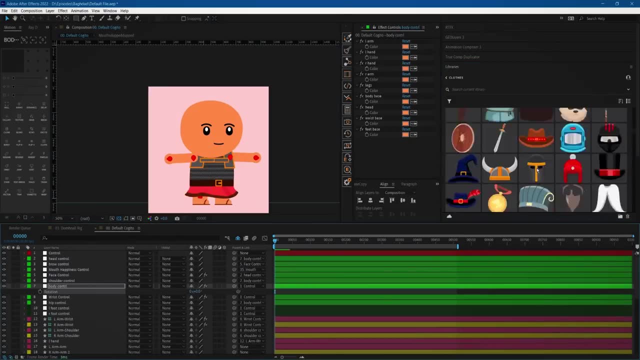 last year I used this app to animate everything. Now I use this PC, whose name, by the way, is Earp. Adobe After Effects looks scary and complicated, and it can be, But you control it essentially using 3 things: Keyframes, layers and effects. 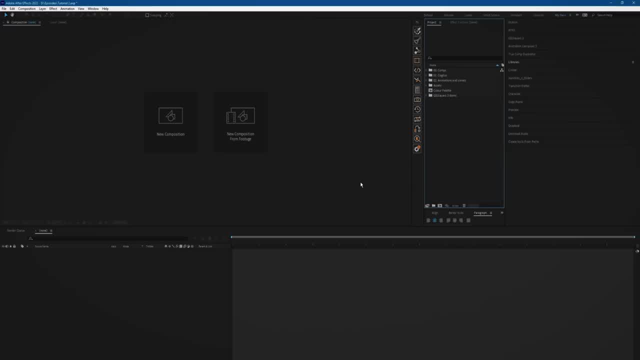 and effects. That's it. Let's make a ball bounce. for example, First you make a composition which is After Effects version of a scene. I make my compositions 1920 by 1080 at 60 frames a second, but 24 is normal for animation and 30 is normal for video. Let's make a nice background by double. 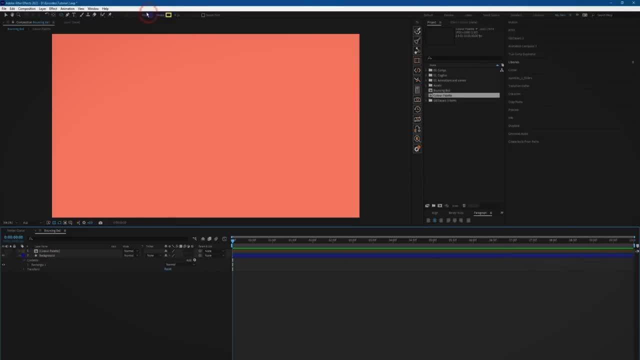 clicking on this rectangle tool and then I'll give that a nice color. Now we make a ball using the same tool, but switching it to a circle. We'll hold down shift while we drag, which will make a perfect circle. All we have to do now is click on our ball layer, twirl down to its properties, click on this. 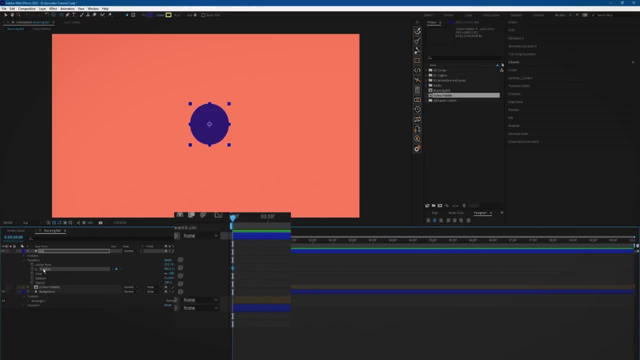 stopwatch on the position property, which will create a keyframe. Keyframes are the start and end points of animation. If you keyframe a ball's position layer here and then move ahead a few frames and put another keyframe here, it tells After Effects to start moving at this moment in. 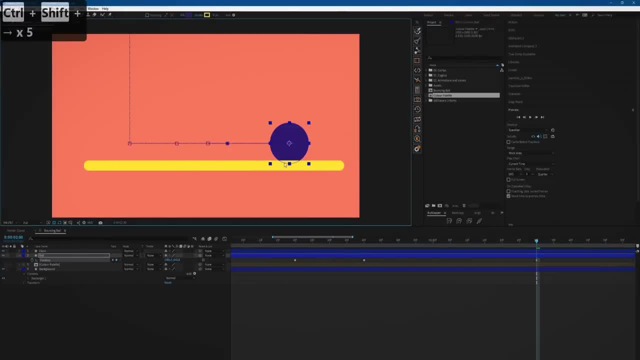 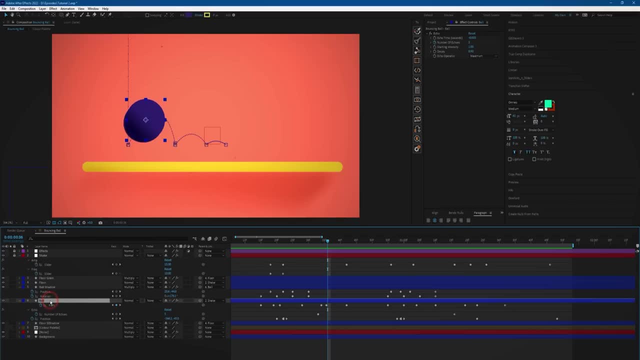 time and end. at this moment in time, We can add a few more keyframes to give this ball a little more life, tweak this composition a little bit and all of a sudden I have an okay looking animation. If I don't like the color of the ball, I can add a few more keyframes. 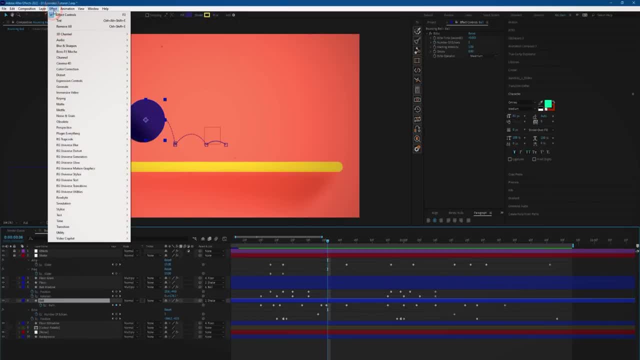 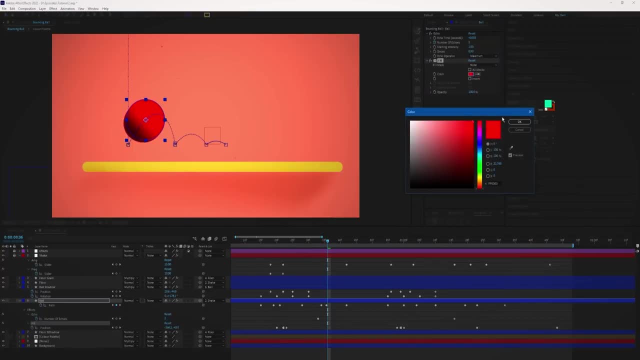 If I don't like the color of the ball, I can change it here, or I can go to effects up here and then click on fill, which adds an effect that fills this layer with a new color. So that's how After Effects works: Layers, keyframes and effects. For my maps, I use an After Effects plugin called Geolayers and 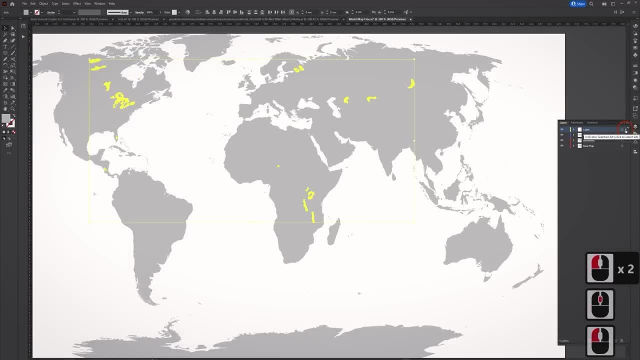 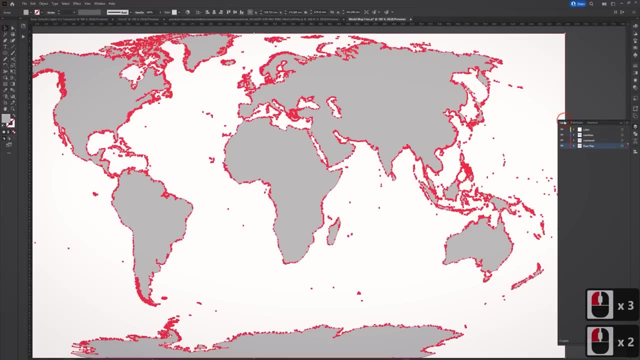 have for years, but it is fairly expensive. Before that, I made my own maps. There are tons of free maps on Wikipedia that you can download and then customize in Illustrator or Inkscape. I have a giant vector map with every single country in the world cut out. If you want to see how I do that. 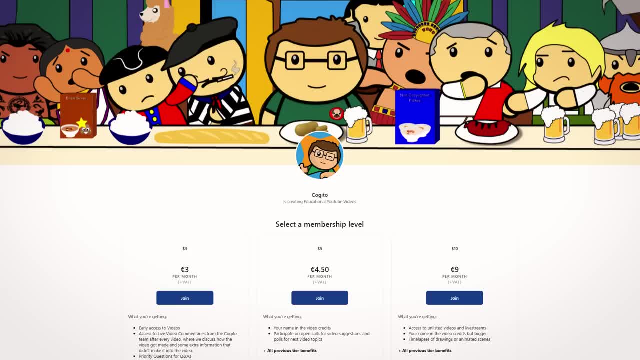 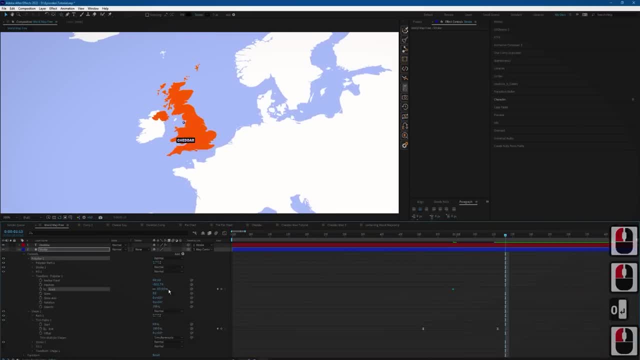 you can download it. it's up on my Patreon and over the next few days I'll be uploading in depth tutorials to my Patreon on how I animate my cogitos, motion graphics and maps in both the expensive geolayers way and the freeway. For my cogitos I have a complicated rig setup that I've 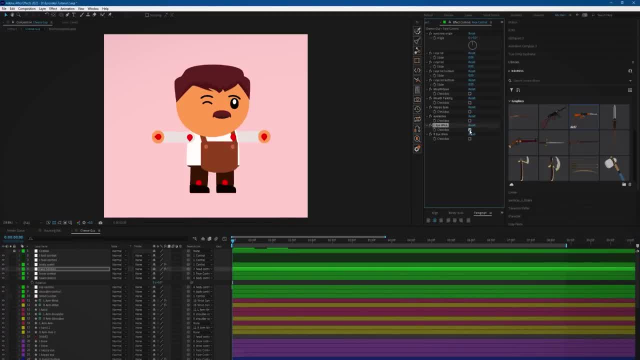 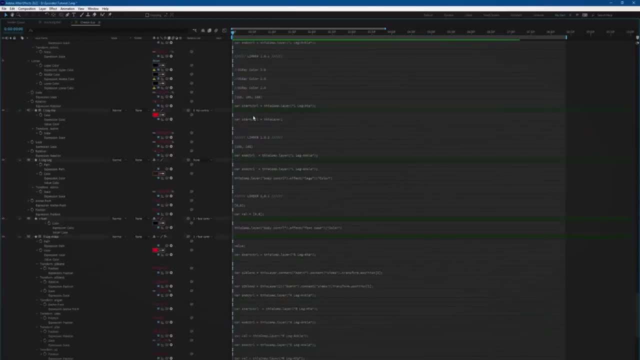 been tweaking for years. I have all sorts of controls for small details like winks, surprised faces, blinks, arm over body transitions, and I use a good amount of code to handle some of this. I also use a plugin called Limber, which costs money, and this handles the arm over body transitions. 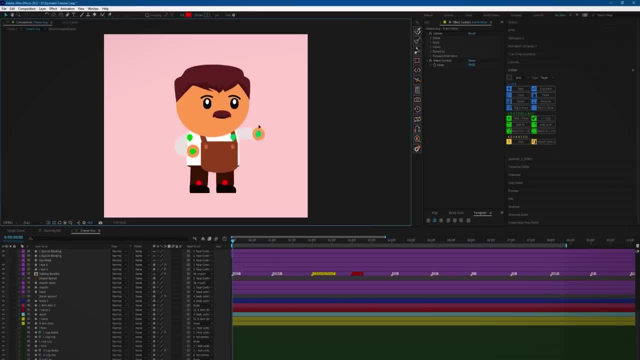 you see in the image, and I use it to handle some of this. In the meantime, I also use a plugin called Limber, which costs money, and this handles the arm over body transitions which I will be working on arms and legs. This plugin just speeds up the process so I don't have to animate every 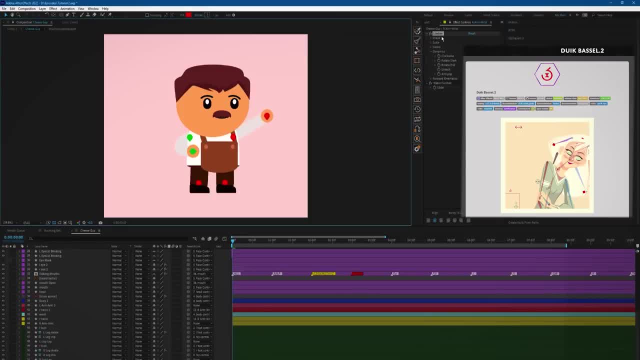 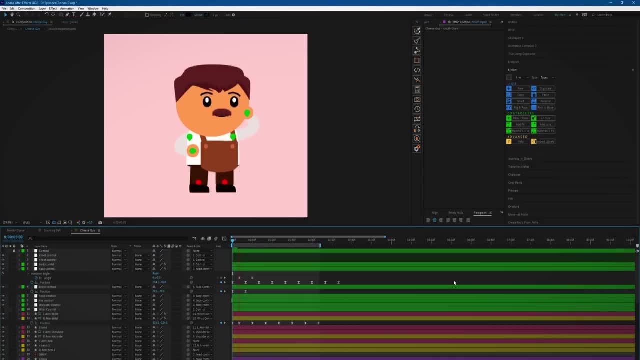 single elbow and knee bend. You can use a free tool called Duik, which is very similar, To make a cogito wave. all I have to do is select a wrist keyframe. it make some more keyframes as I move it back and forth. and now he lives. 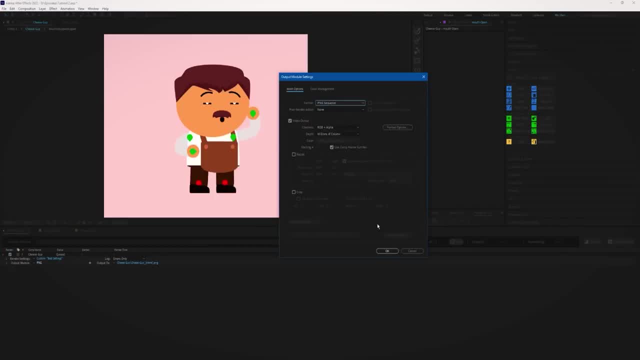 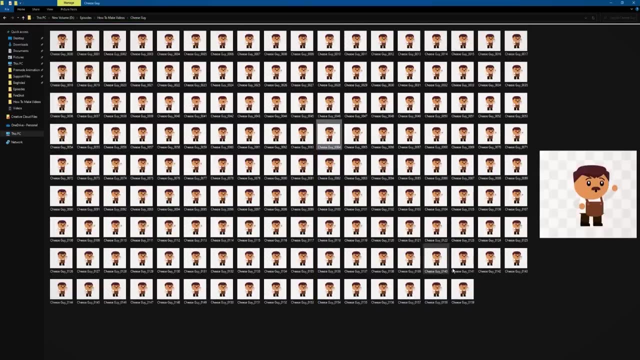 Once I'm done, I render everything out as a PNG image sequence. I do this because an image sequence saves every single frame as one picture, So if After Effects crashes- which it does a lot- I don't lose everything and just have to render from the last saved. 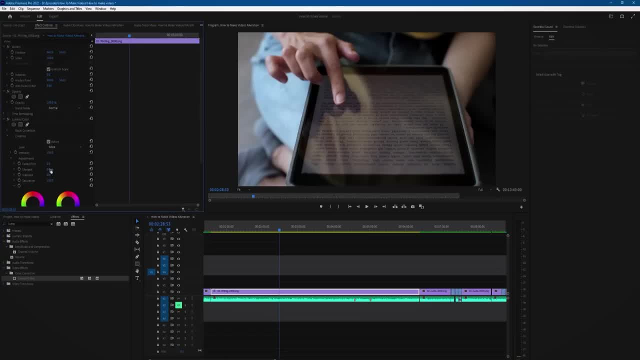 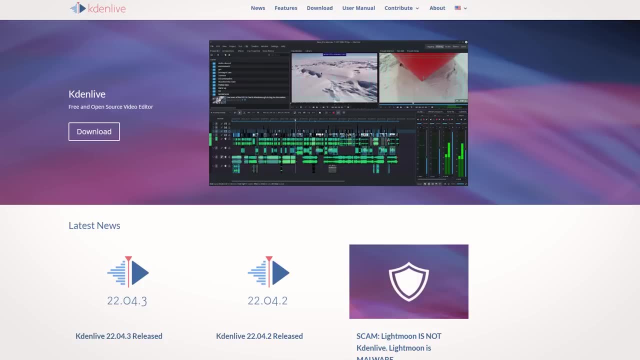 picture file Editing and music. I use Adobe Premiere Pro for video editing, but when I started I used Kdenlive, which was eh, but it was free. Another alternative to Premiere Pro is DaVinci Resolve, which is free and apparently very good. I don't actually have to use this program much. 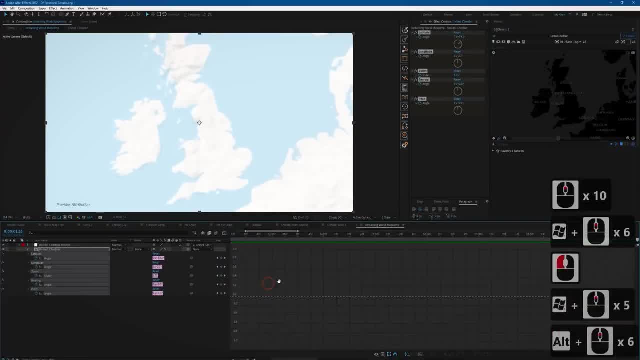 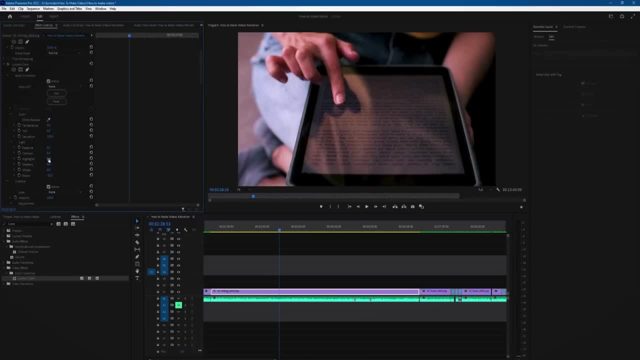 because, as an animated channel, most of my editing is done in After Effects. In Premiere I mostly just tweak some colours, add some transitions, re-organise the scenes, slice slightly and then add sound effects and music. I use Epidemic Sound for music and sound effects. 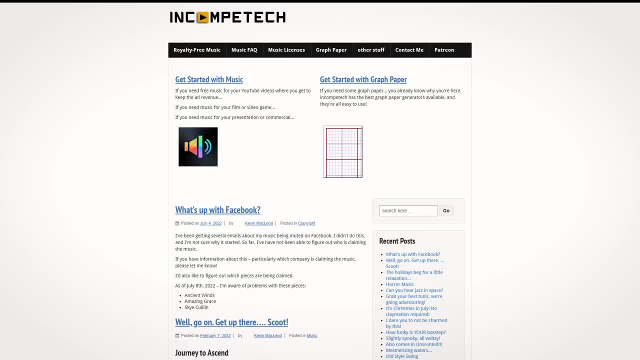 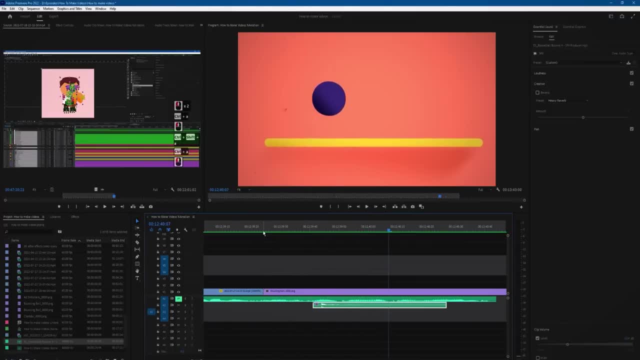 but Kevin Macleod has a bunch of free music on his site and he is essentially the soundtrack for most of YouTube. I add whatever sound effects I think will sound nice. I lower the volume so that they're not super annoying, and then the music I also lower to around. 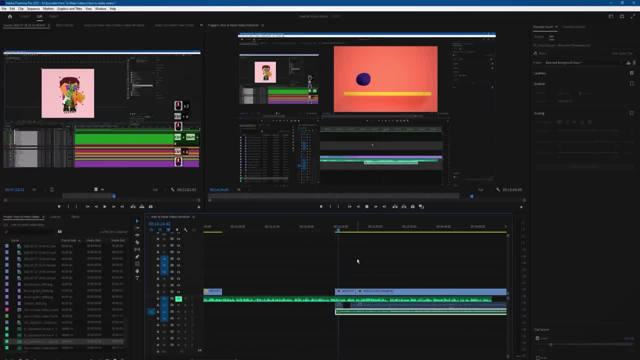 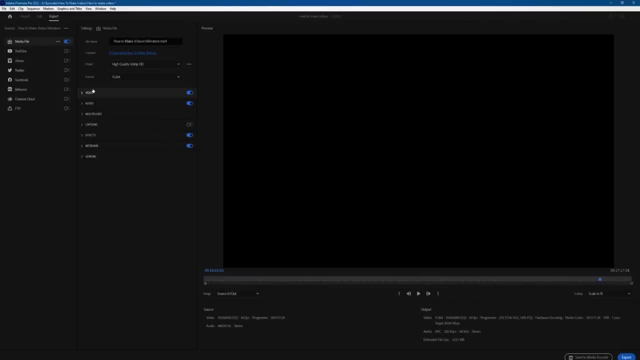 negative 28 decibels. I want the music to be there, but I don't want it to be overwhelming. Once I've done all this, I go to export and I render my video. These are the render settings that I use. I'm not sure if they're good, but the videos look ok. I assume. Add all this. 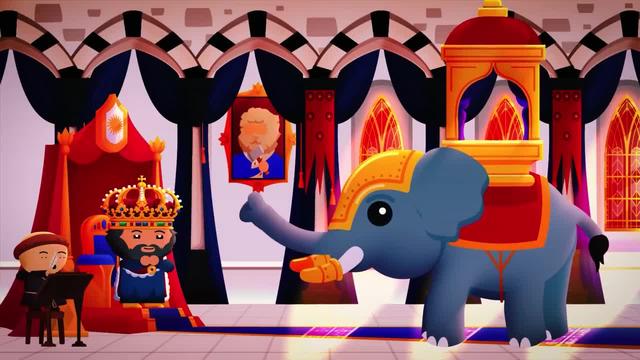 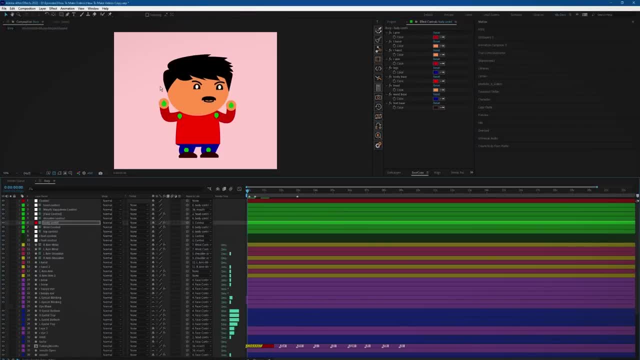 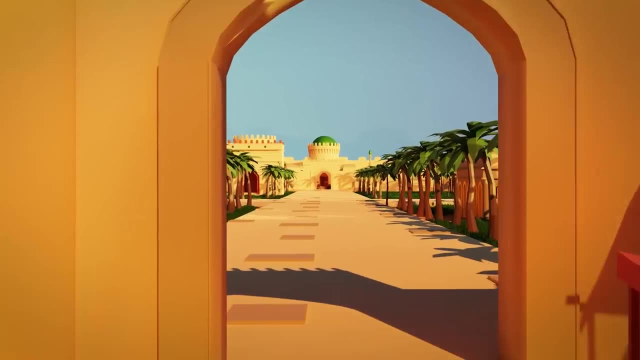 together and you've got an educational video. All of the tools that I showed you today are pretty complex, but with a little bit of effort you can master them. I started off making videos that looked like this: The only way I progressed to make videos that looked like this is by following tutorials and courses.